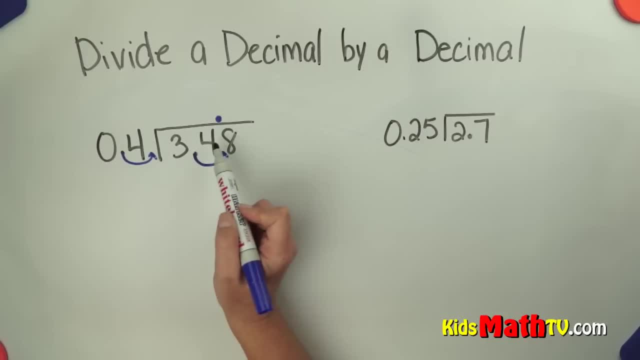 So there are no fours in three, but there are eight in 34.. Eight times four is 32.. Subtract, I get two. Bring down the eight. How many fours are in 28? Seven, Seven times four is 28.. Subtract and we get zero. So three and forty eight hundredths divided by four tenths is eight and seven tenths. You can actually check your division by. 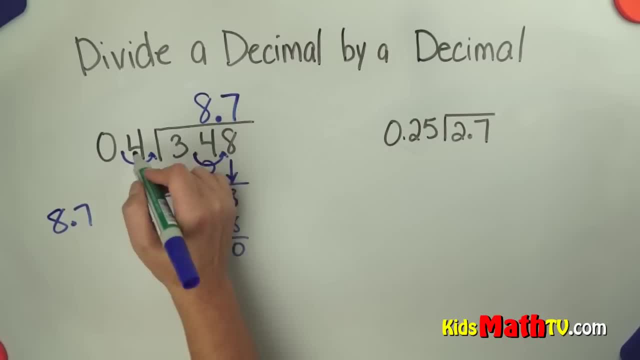 multiplying. We take our answer, eight and seven tenths, and multiply it by four tenths, We should get three and forty eight hundredths. Let's see 28,, 32,, 33,, 34.. And I see one, two decimal places in my problem. So I need one, two decimal places in my answer. So we get the same answer. Three and forty eight hundredths was my divisor. 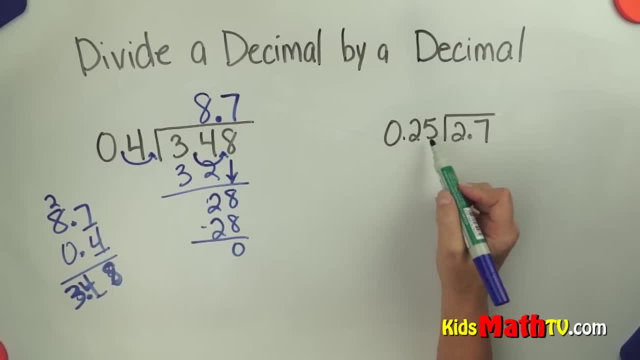 Okay, Let's try this one. In this one, I see two decimal places in my divisor, so I need to move it over two places to the right As far as I can go, Which means I have to move this one over two places as well. 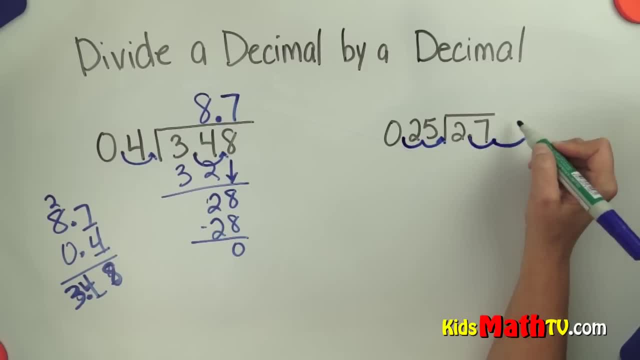 Well, there's only one number there, but right here is a placeholder zero. So now my decimal is here. I moved it two places- two places in my divisor, So two places in my dividend- and bring it straight up. And now I divide How many 25s in 27? 1. 25.. I can subtract and bring. 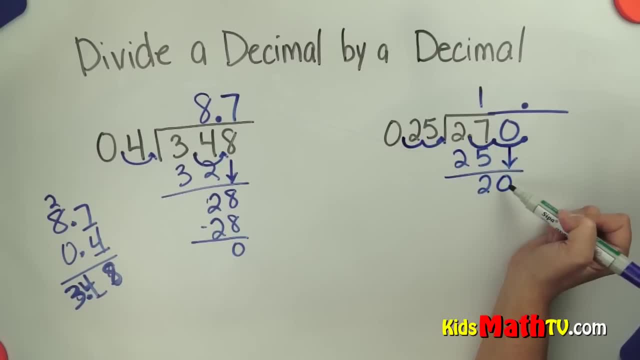 down a 0.. How many 25s in 20? Well, there are none. That's 0.. Subtract is 20.. Now I can put another 0 here and bring it down, making 200. So I can addend zeros after a decimal. How many 25s in 200? Well, 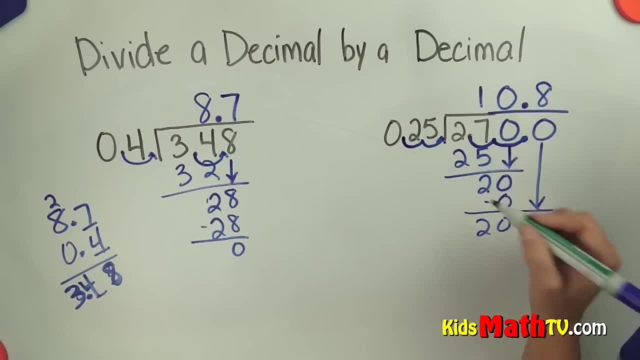 that is 8.. 8 times 25 is 200. Or 8 quarters, if you're thinking money, And 0. So 2 and 7 tenths divided by 25 hundredths is 10 and 8 tenths And that's the end of our. lesson. Lesson on dividing a decimal by a decimal.